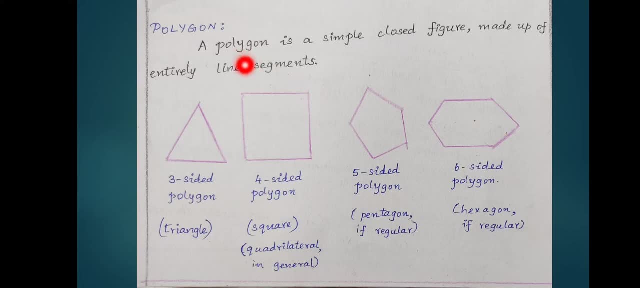 So a polygon should be a simple closed figure, but with a condition. What is the condition? That figure should be made up of completely line segments. You should not use any curves to make a polygon. See, we have a 3 sided polygon, 4 sided polygon, 5 sided polygon, 6 sided polygon. You can draw 7 sided, 8 sided polygons also, as you wish. 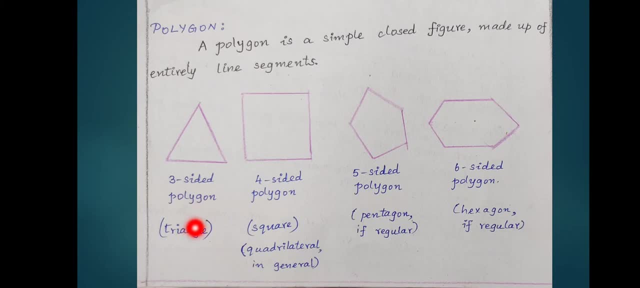 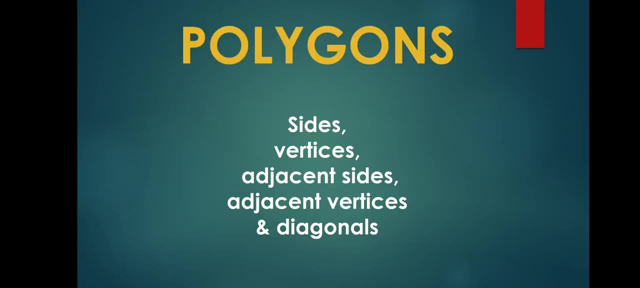 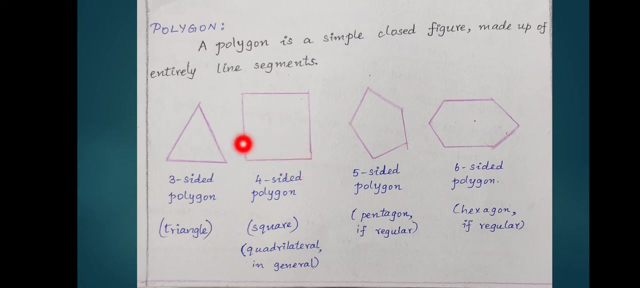 3 sided polygon is called triangle. 4 sided polygon is called quadrilateral in general, If all the sides are equal, then it is called a square, And all the angles should be 90 degree. So there are some conditions to get a square from a quadrilateral. 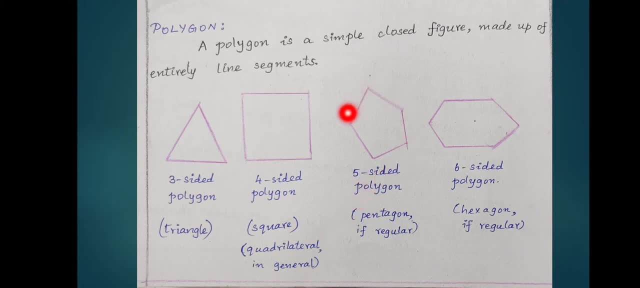 Similarly, if all the sides of a 5 sided polygon are equal, then that 5 sided polygon is called regular and it will be called a pentagon. And if all the sides of a 6 sided polygon are equal in length and all the angles are equal, then it is called a pentagon. 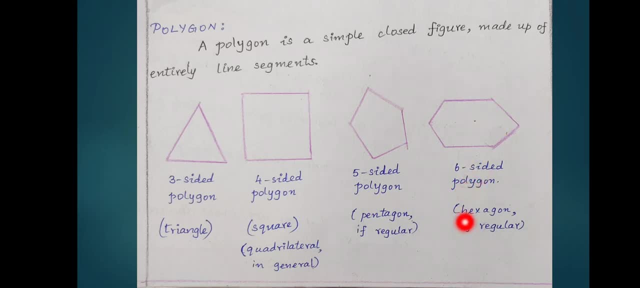 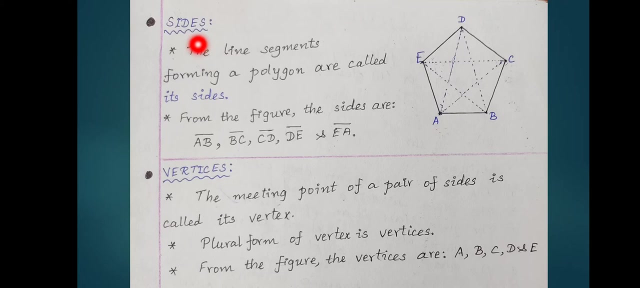 That 6 sided polygon will be called as a regular 6 sided polygon, and so it will be called as a hexagon. Next sides: Sides of a polygon. The line segments forming a polygon are called its sides. See, we have a polygon. 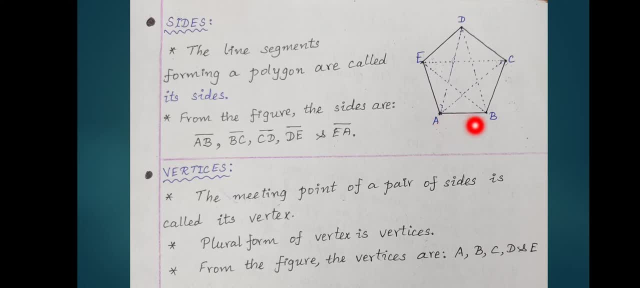 We have a polygon here with 1,, 2,, 3,, 4, 5 sides. What are the line segments forming this polygon? A, B, C, D E. A, B, C, D, E are the 5 points. 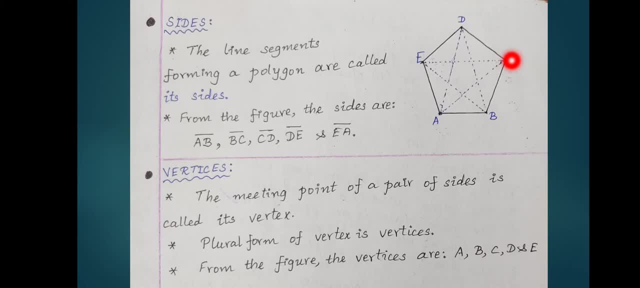 A, B line segment B, C line segment, line segment C D, line segment D E and line segment E A are the sides A, B, C, D, E are the 5 line segments which form the polygon A, B, C, D, E. 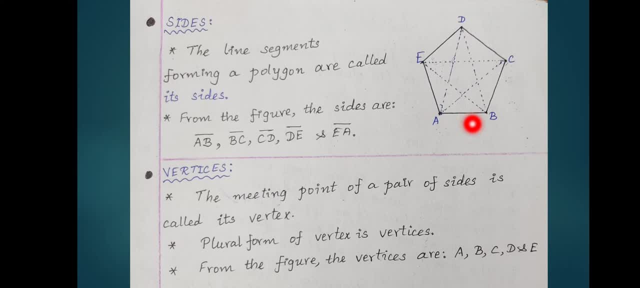 Also, these line segments are called sides of the polygon. Now, what are the vertices of a polygon? The meeting point of a pair of sides is called its vertex. If so, what do you mean by vertices? Plural form of vertex. 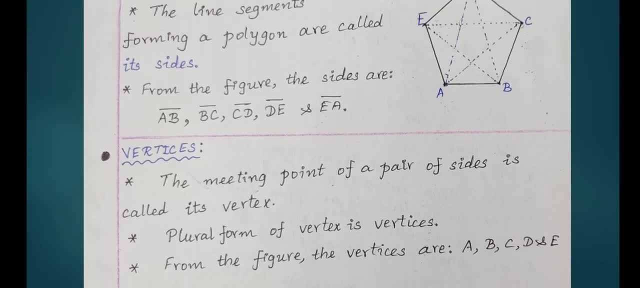 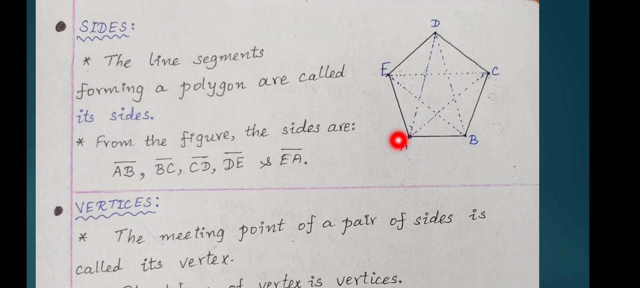 Vertex is vertices. So listen, Sides are line segments, Vertices are meeting points. See from the figure the vertices are A, Because this is the meeting point of line segment E, A and A, B. Next vertex is B. 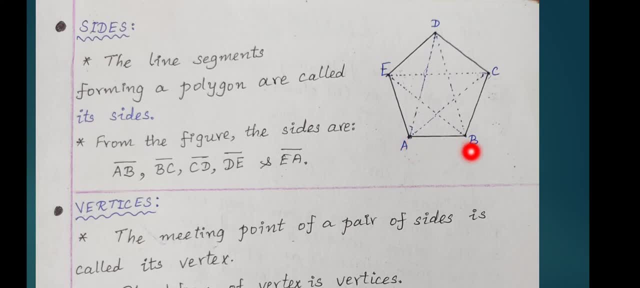 B is the meeting point of A, B and B C. B is the meeting point of A, B and B C. C is the meeting point of B, C and C D. D is the meeting point of line segment C, D and D E. 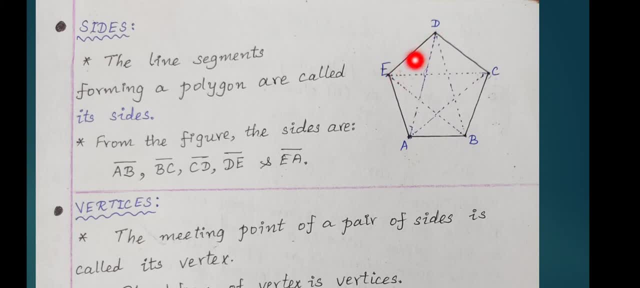 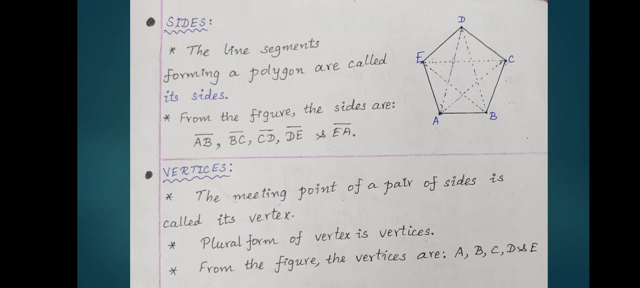 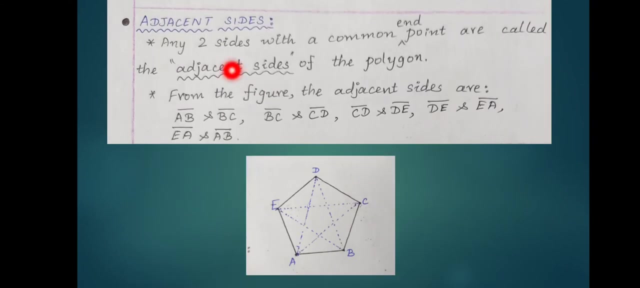 E is the meeting point of line segment D, E and E, A. So A, B, C, D and E are the vertices of the polygon A, B, C, D, E. Okay, Adjacent sides. Adjacent means next. 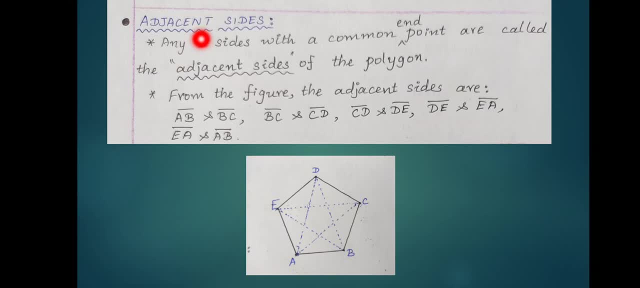 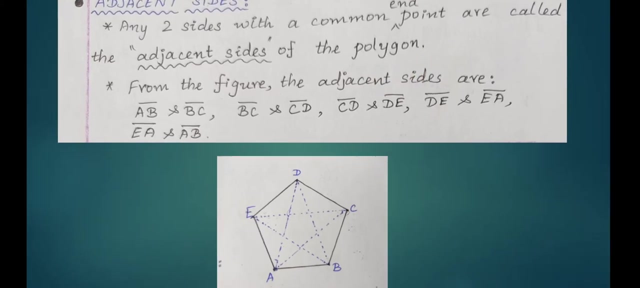 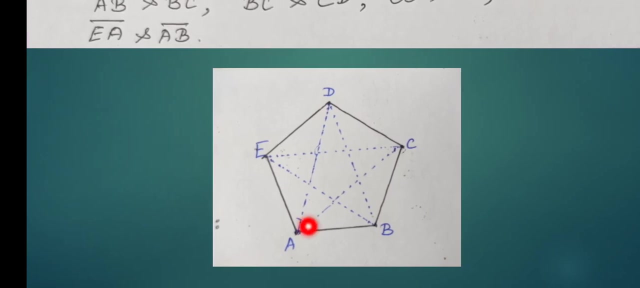 Let us see the definition. Any two sides with a common end point are called the adjacent sides of the polygon. So take any two sides with one common point, Consider, Consider A, B and B C: They have the common point B. 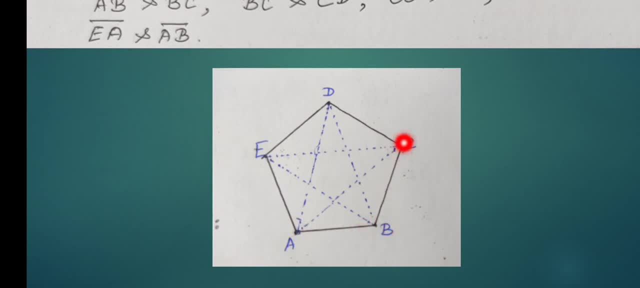 So the sides A, B and B C are called adjacent sides. Similarly B C and C D have the common point C. So line segment B, C and C D are the adjacent sides. Similarly C D and D A have the common point C. 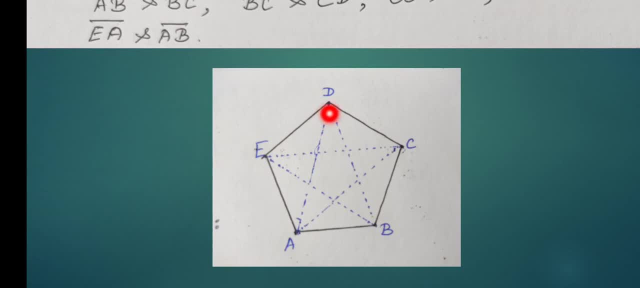 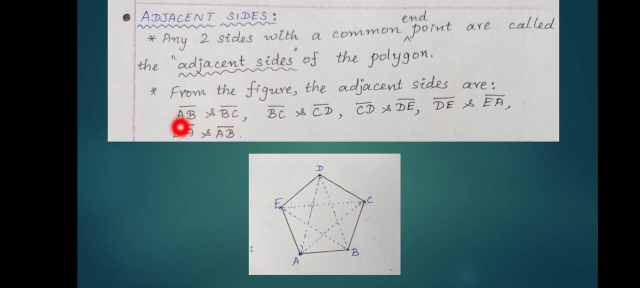 C, D and D- A have the common point D, So they are adjacent sides. D, E and E A are adjacent sides. E A and A- B are adjacent sides. Since the sides are line segments. we denote a small line above A- B. 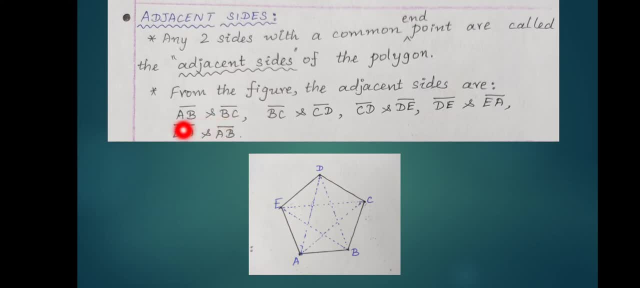 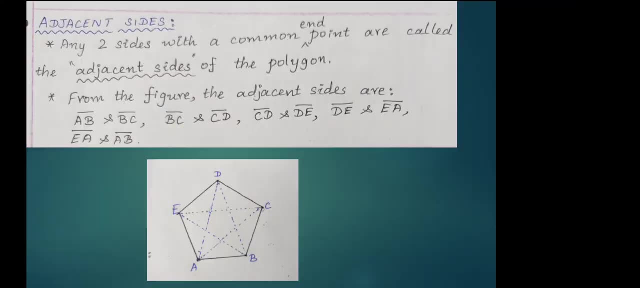 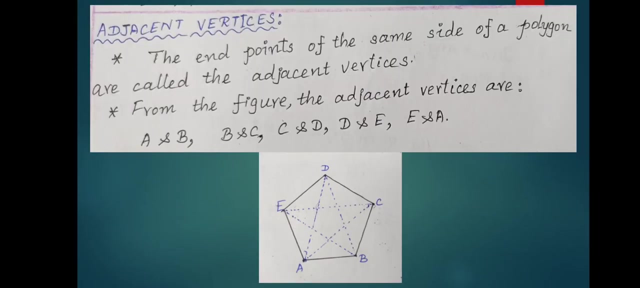 Okay, We should read it as line segment A B and line segment B C. Okay, Adjacent vertices. The end points of same side of a polygon are called adjacent vertices. See Consider any one line segment. You will get two end points. 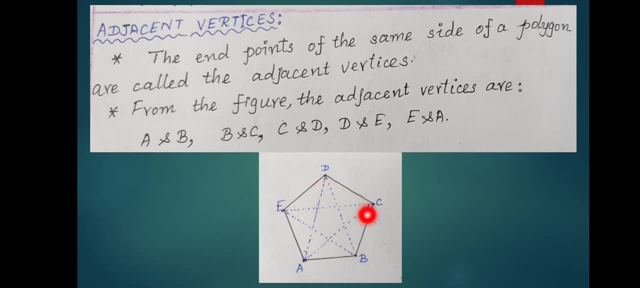 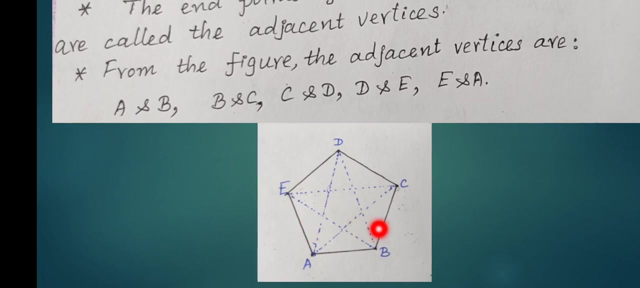 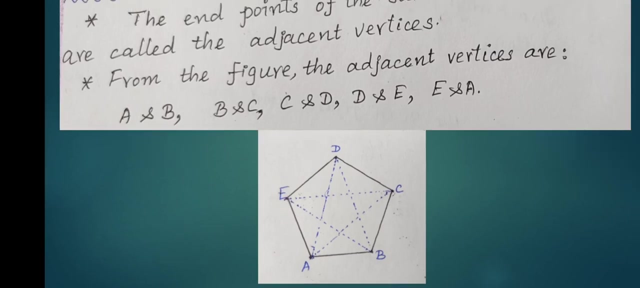 These end points are called adjacent vertices. One vertex is next to the other. Okay, So from the figure, adjacent vertices are: A, B, B and C, C and D, D and E and E and A. Okay, Remember, vertex is the meeting point. 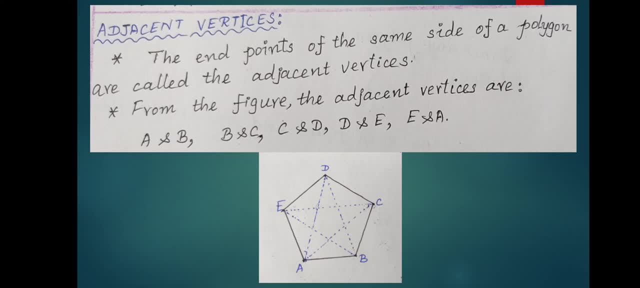 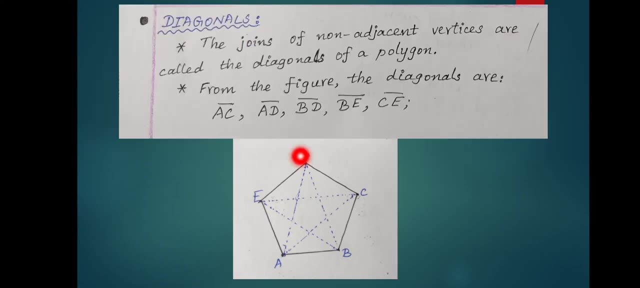 And side is the line segment. Okay, Diagonals: The joints of non-adjacent vertices are called the diagonals of a polygon. You know very well, plural form of vertex is vertices, Non-adjacent If two vertices are next to one another. 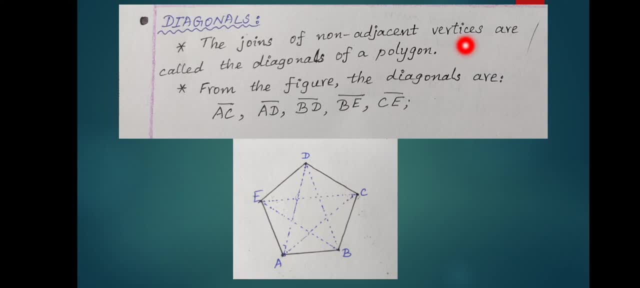 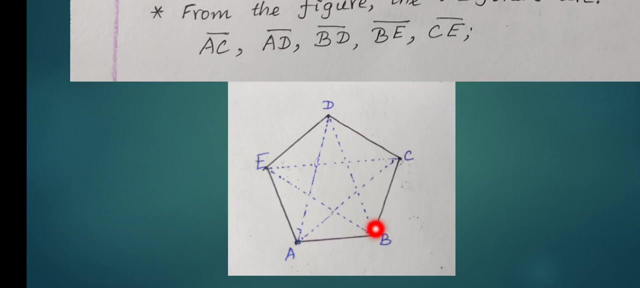 they are called adjacent. If two vertices are not next to one another, they are called non-adjacent vertices. Okay, The joining line segments of those kind of vertices are called diagonals of the polygon. From the figure you see, A and B are adjacent vertices.